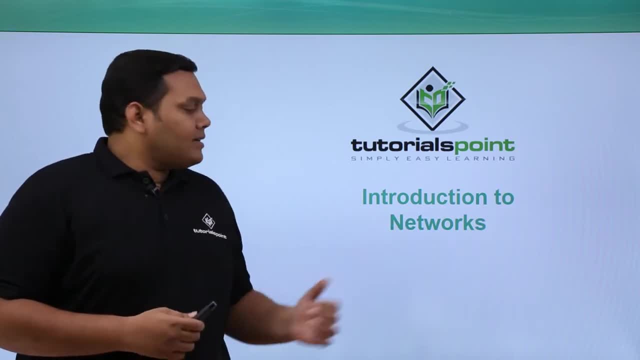 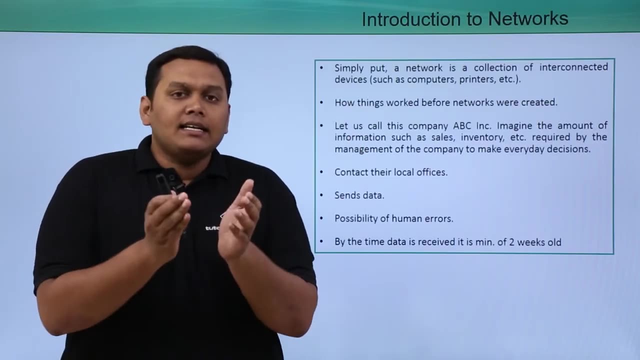 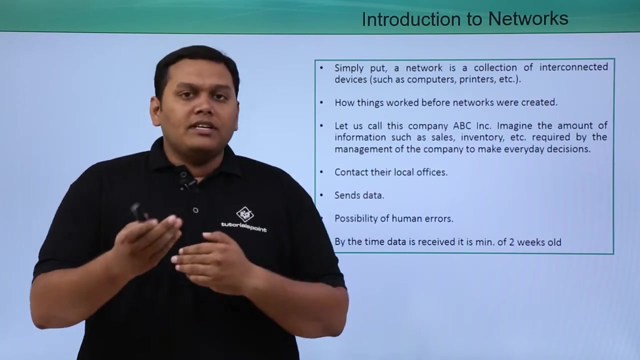 In this video we are going to discuss about introduction to networks. So what is a network? By simply you can say network is a collection of interconnected devices like computers, printers, etc. So how things work before networks we will be discussing. 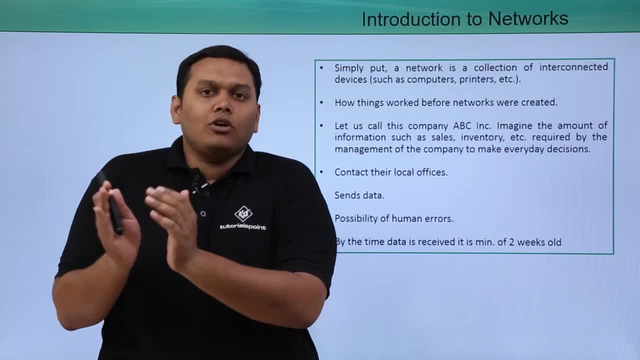 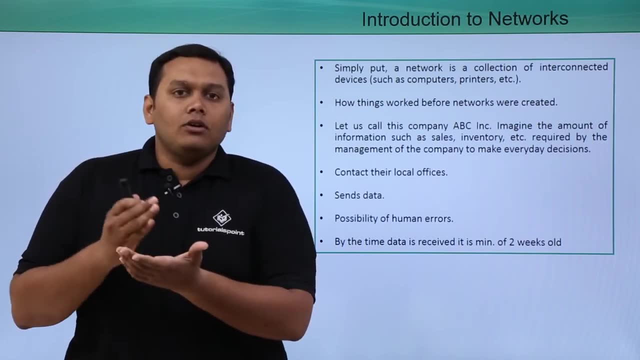 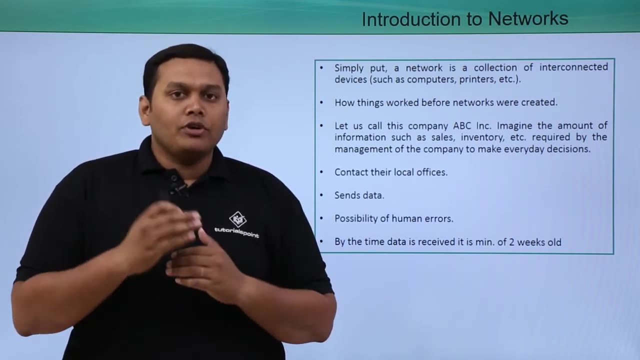 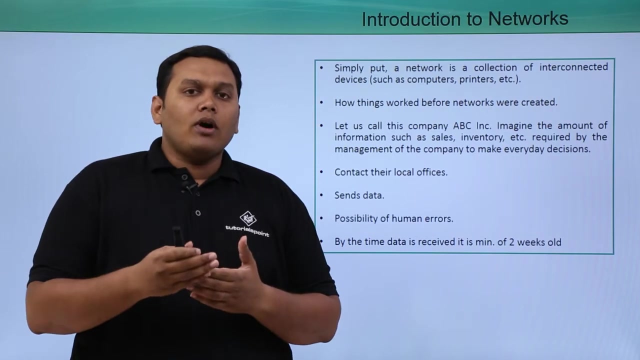 So before networks got introduced, what is the situation or scenario? So better take a best example of ABC Incorporation Company, which has multiple local offices located in Singapore, Australia, India, USA and UK. So here you see the information generated by sales, inventory etc. departments has a lot of information so that they have to send this information to the management. 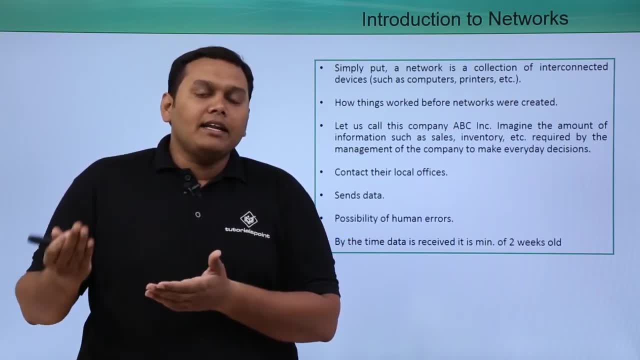 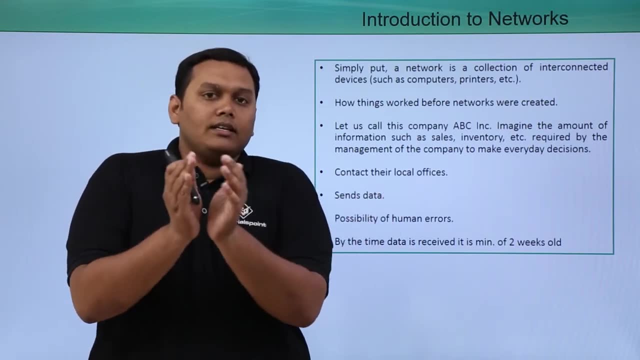 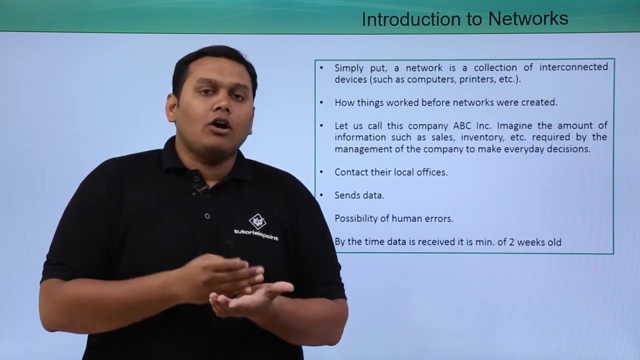 So the management can take day to day, everyday decisions here. So imagine how they contact their local offices. So a headquartered it is in USA, so the management, which is sitting in USA, request information of different departments in all the local offices to their head office. 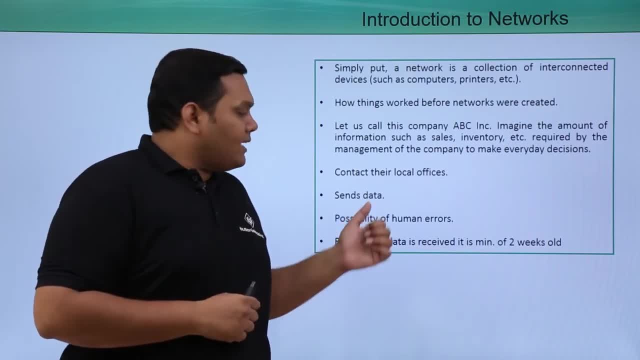 And you can see about the head office details. they will be sending the data through mail- mail in the sense post mail. So here, after sending the information through post, the data will be two weeks old. So here, after sending the information through post, the data will be two weeks old. 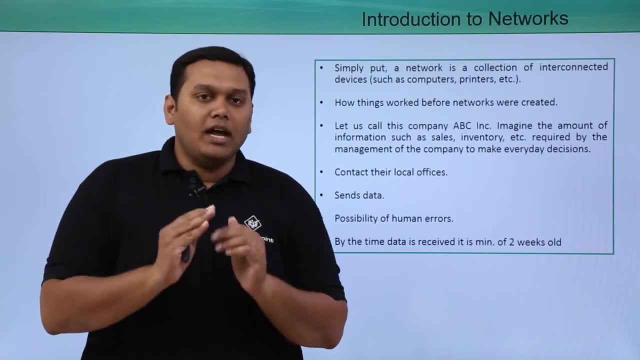 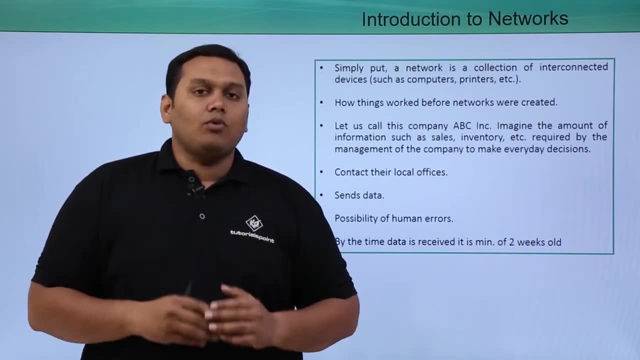 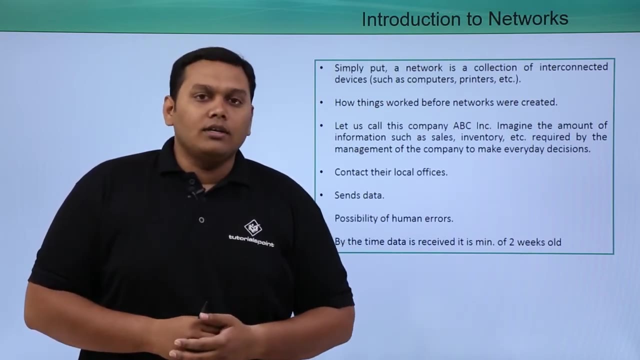 and also possibility of human errors will occur. so different departments and different local offices will send the information to the management sitting in the headquarters, so that after requesting the data and after the data is received it is already two weeks old, so here there is a possibility of human. 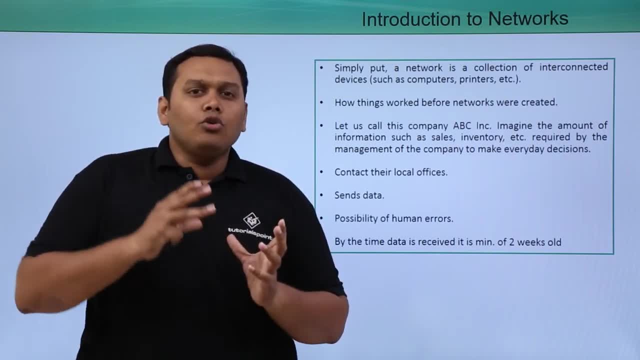 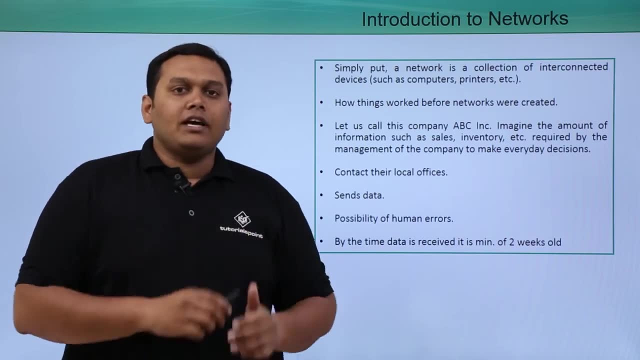 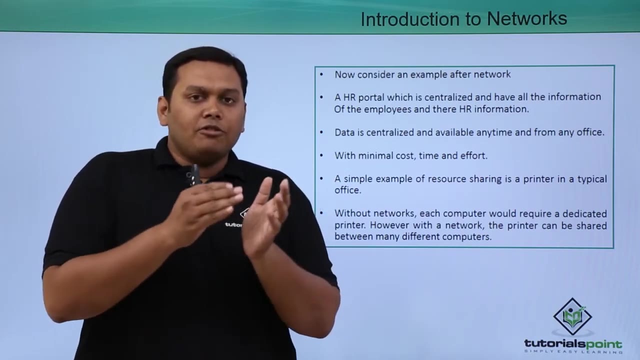 errors and also the decisions might be pending and no growth or no productivity of the company will be forwarded to the next year. so in the next scenario, imagine the same example, considering the network in place. so the ABC information or the ABC information is available in a HR portal. so imagine example of a HR. 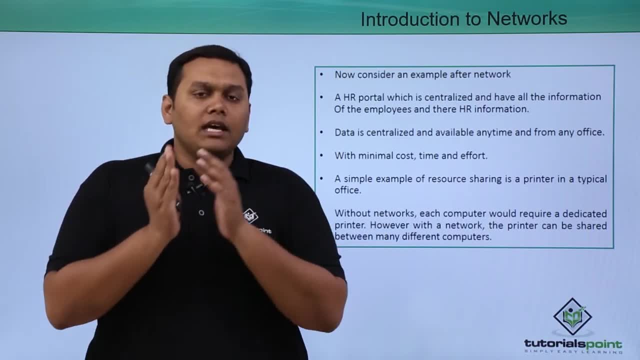 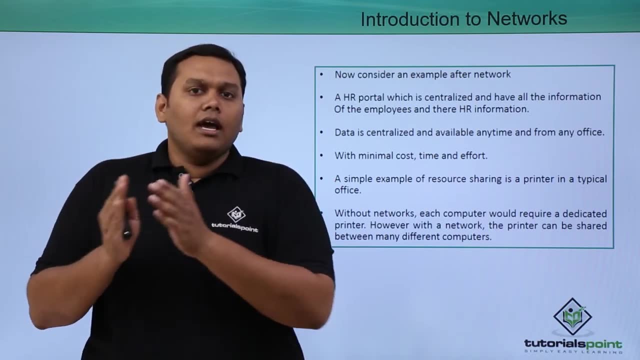 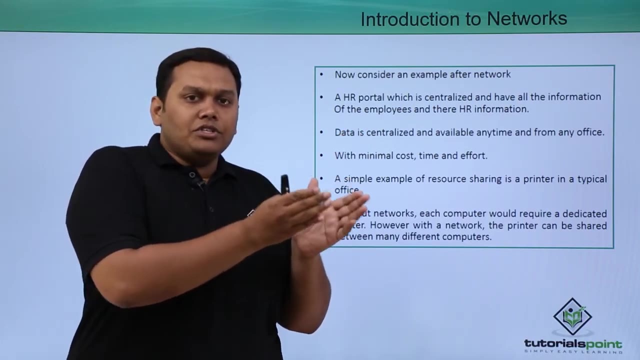 portal which is having information of all the employees coming into the, joining the company or leaving the company in a HR portal: different local offices and different departments. the HR portal has information so that the person sitting in the management, which is your headquartered in USA, can view a person leaving in Australia and